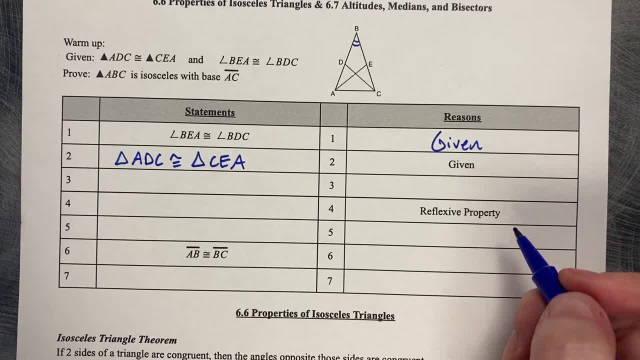 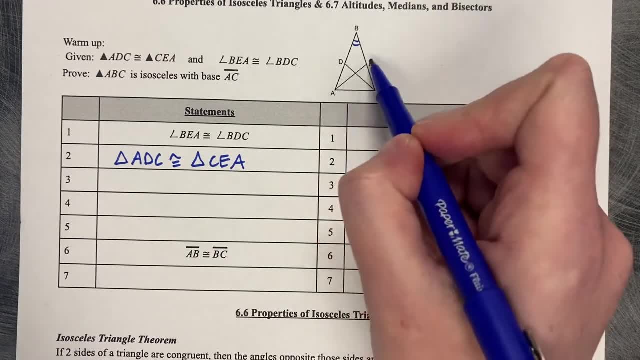 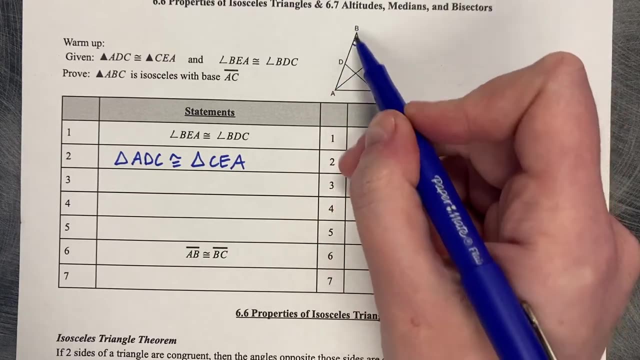 Then our next one is totally blank. but we kind of know what we need to talk about. We know we need to talk about the side links that are congruent between them, because we want to talk about this triangle being isosceles. So eventually I want to talk about AB and BC. 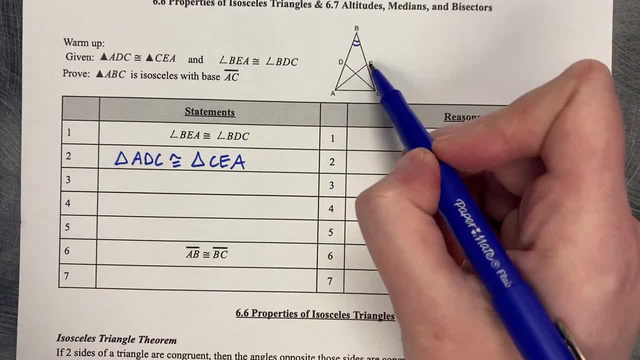 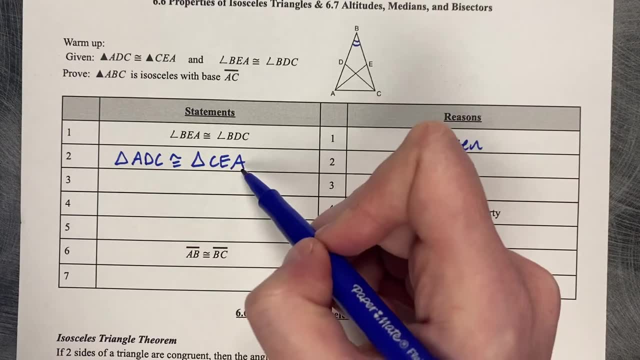 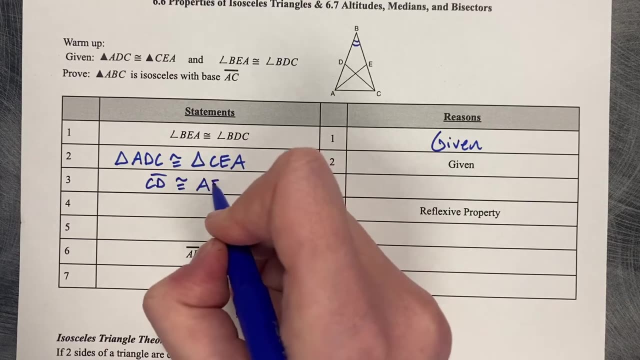 which is down here. We're not quite there. So first thing I want to show is that AE and CD are congruent first, and we know that because these triangles are congruent. So CD is congruent to AE, and that's by the definition of congruent triangles. 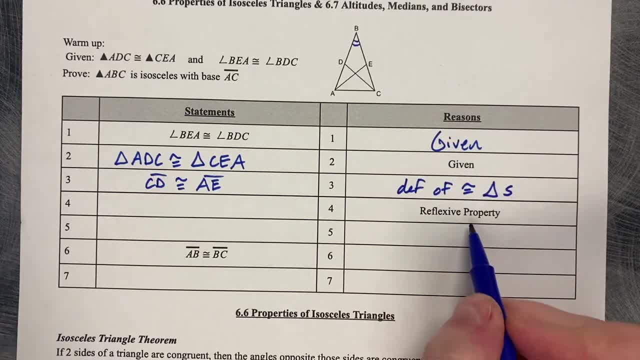 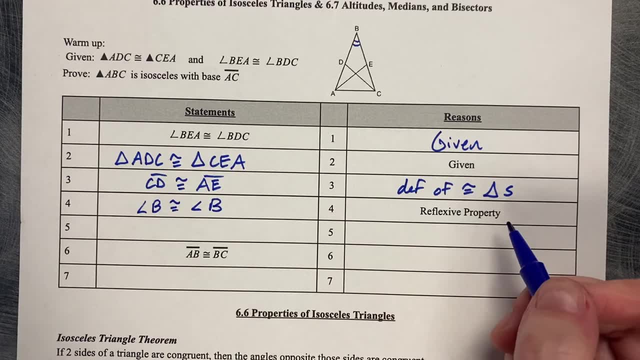 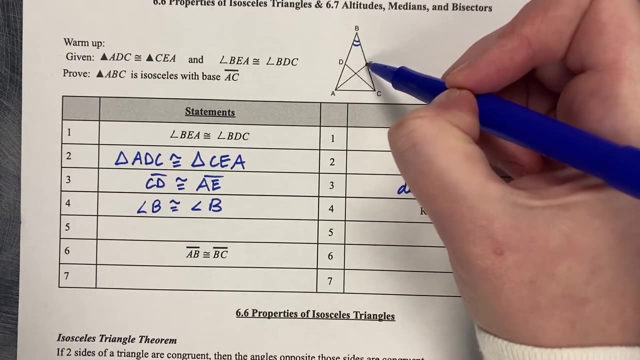 Now the reflexive property. I wanted this angle up here, So angle B is congruent to angle B, And the reason we wanted that is because we wanted to talk about ABE and CBD being congruent triangles. so those top ones. 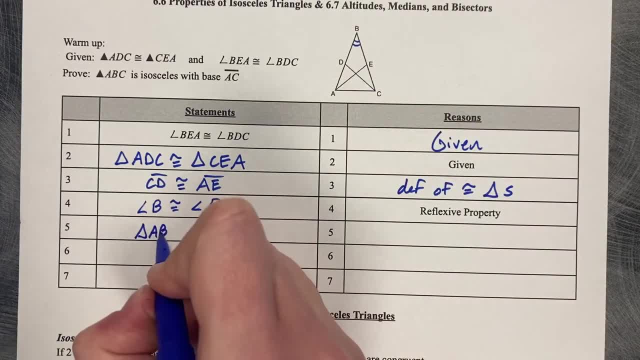 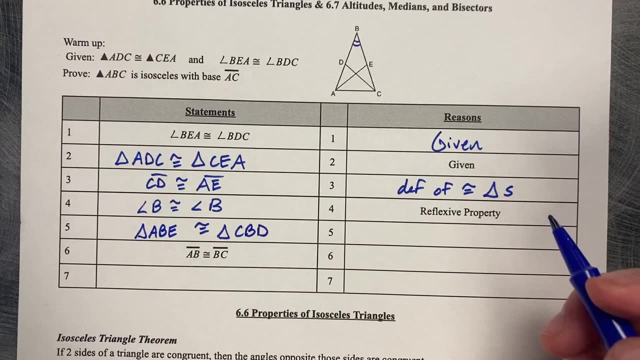 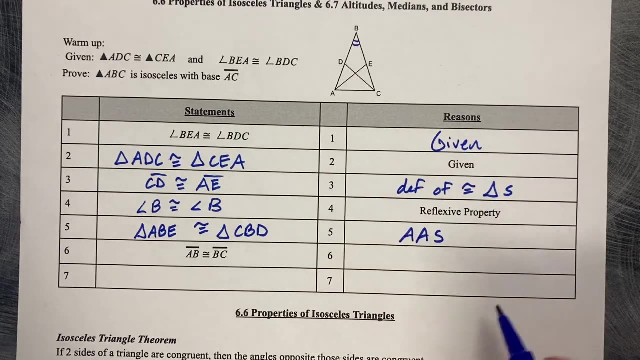 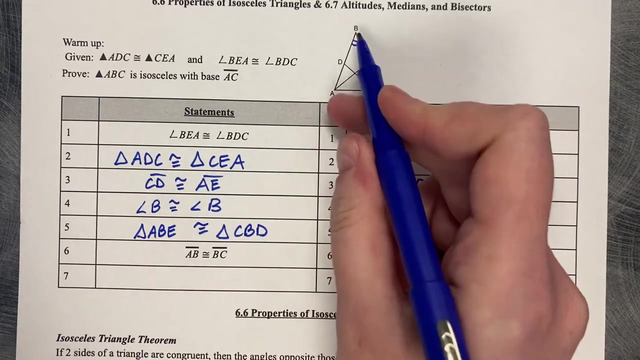 So now we can say that ABE is congruent to CBE, And the reason is because we've got an angle and an angle and a side, Alright. AB is congruent to BC because of the definition of congruent triangles And finally, now we know that ABC is isosceles. 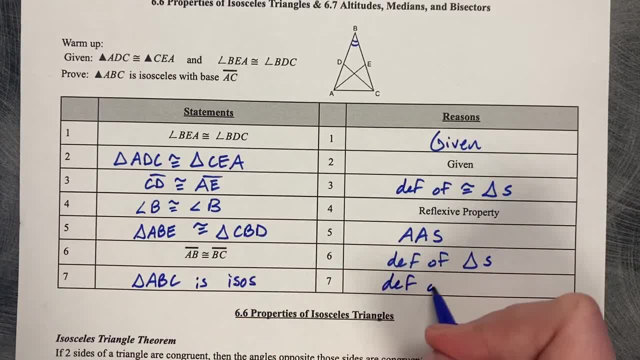 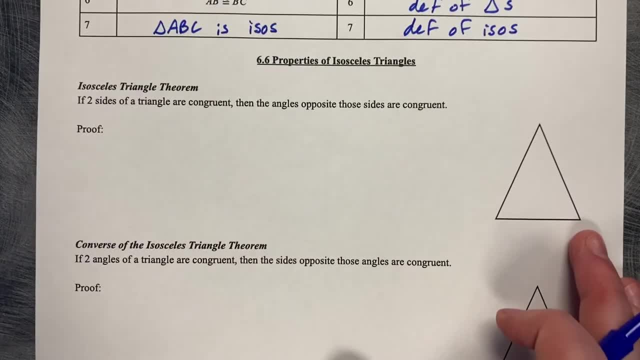 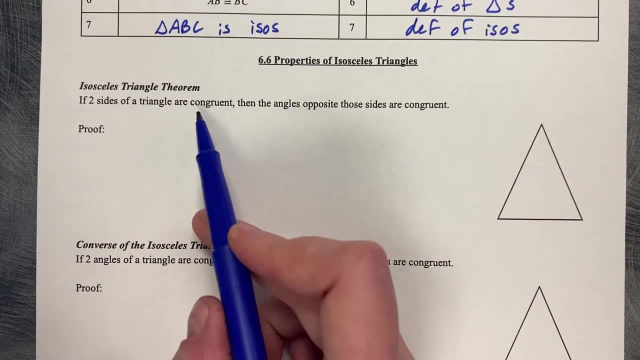 And that's by the definition of isosceles. Okay, 6.6 properties of isosceles triangles. So this is actually the first time we've ever had to do this. but it says if two sides of a triangle are congruent. 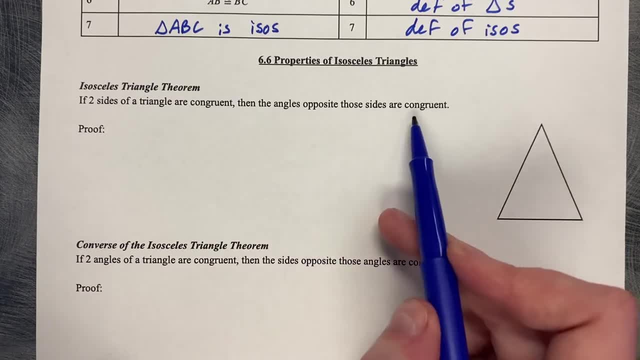 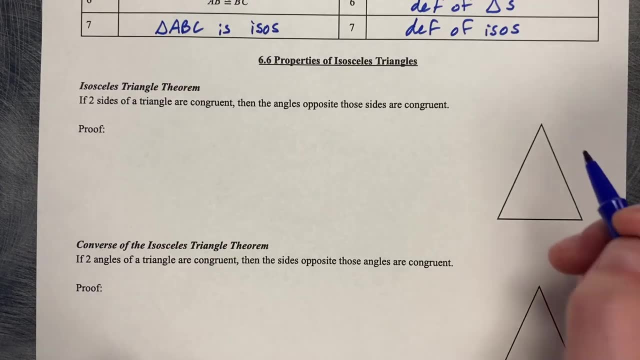 then the angles opposite those sides are congruent. So we've known that to be true about isosceles triangles in the past, but how do you actually prove it? So this is the first time we've had to do something like this. 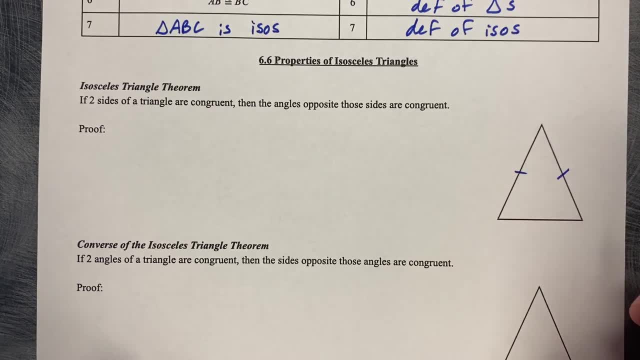 So we know that it's congruent to BC because of the definition of isosceles. We know it's isosceles and that's all we know. It says two sides of a triangle are congruent And what we're trying to prove is that this angle down here. so let's label them. 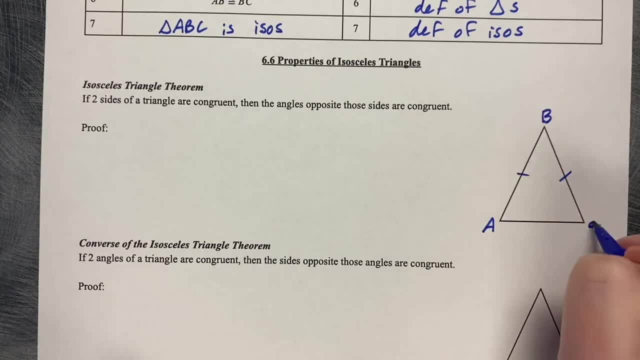 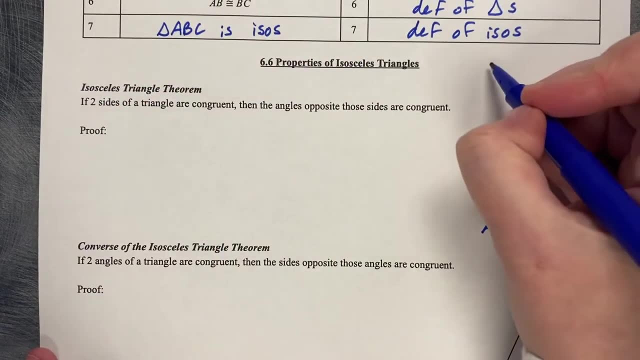 So A, B and C, We're trying to prove that angle A is congruent to angle C. So let's do our given and our prove. I'm going to write it up here actually. So our given is that AB is congruent to BC. 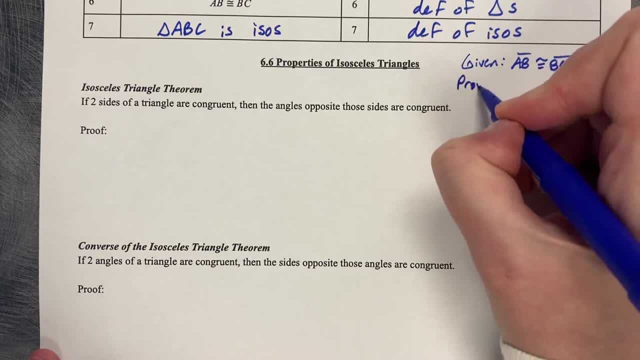 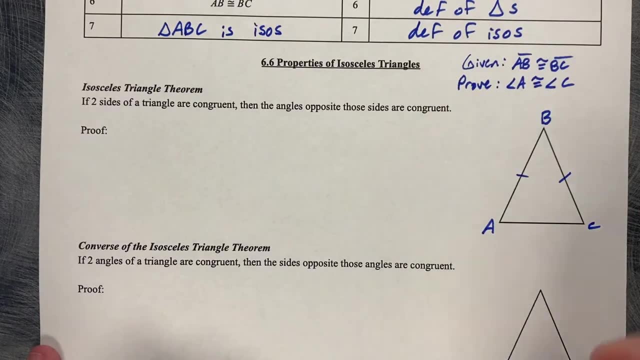 And we're trying to prove that angle A is congruent to angle C. That's what we're trying to show, So this is the first time we've ever had to do this. The trick to this one is to use congruent triangles. 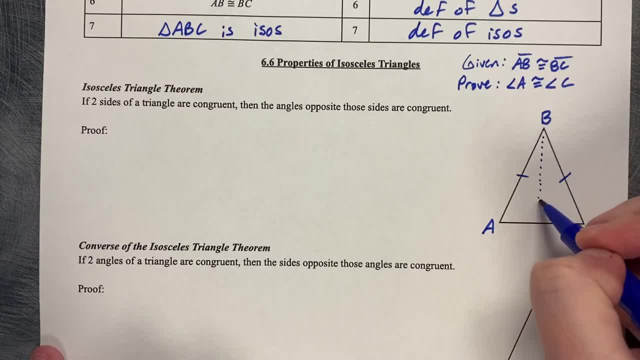 So the first thing to draw in is an altitude, And if you draw in an altitude here, you can say and declare that that altitude is an angle bisector And something we'll talk about in just a minute- well, in a little bit. 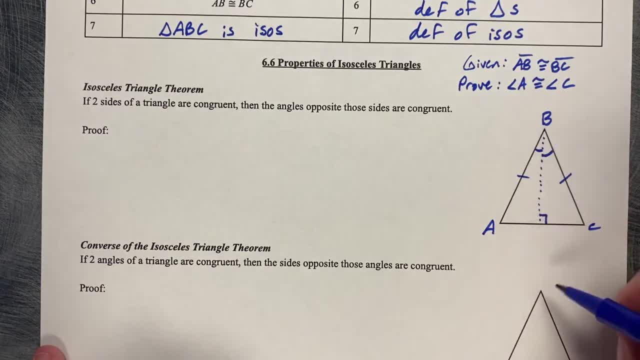 is that, when you draw in this altitude or height of this isosceles triangle, it's also the bisector of AC. We won't need that, though, because all we really need to show here is that I've got a side and an angle. 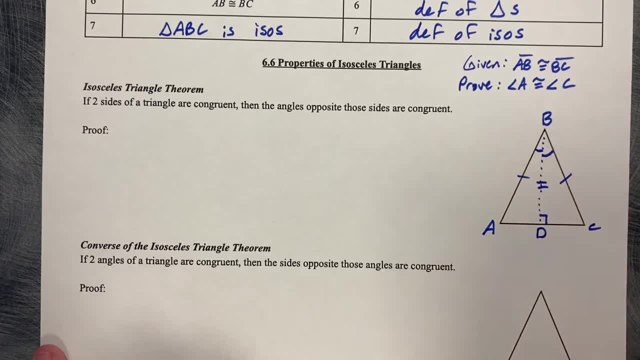 And then this new side link that I drew in BD is congruent to itself. So guess what? we have Side angle side to show that these two triangles are congruent, And thus A is congruent To C. 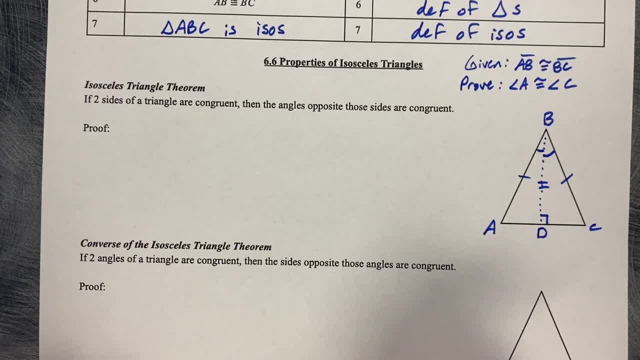 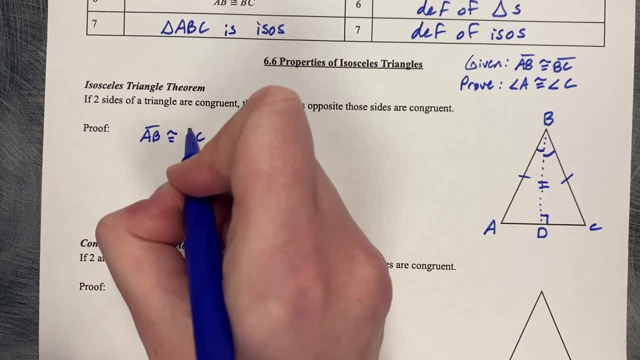 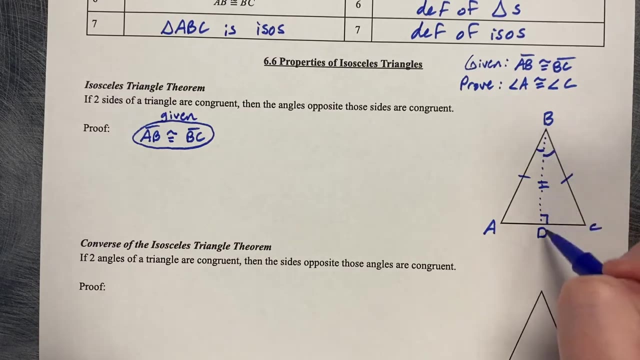 So we're headed towards side angle side. So let's do our given. I'm going to do a flow proof. AB is congruent to BC. That was given. The next thing that I was given or that I added was I drew BD. 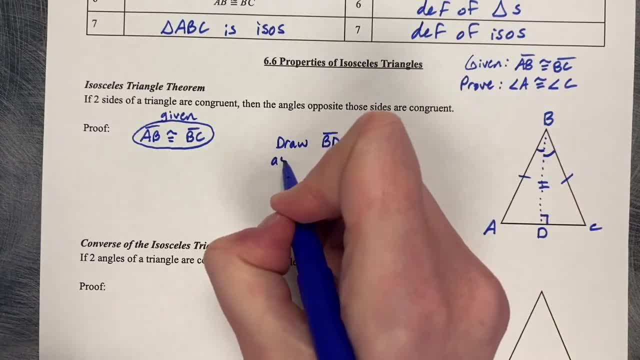 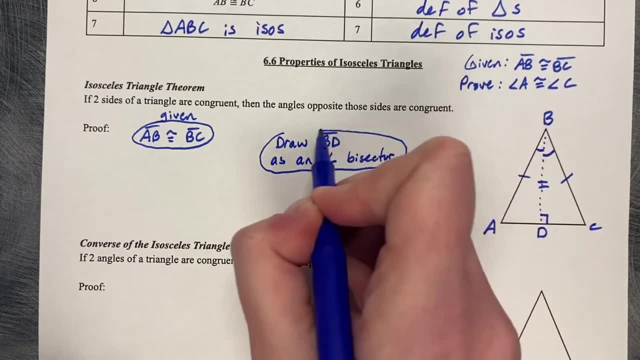 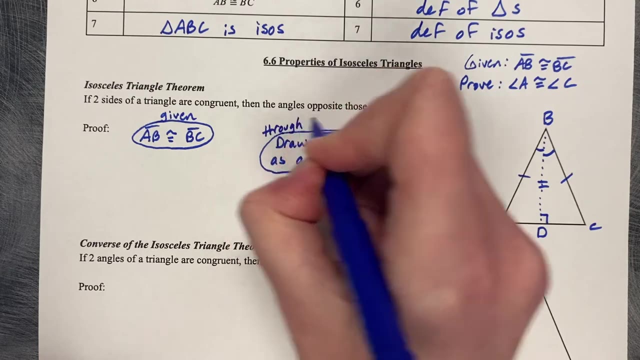 And specifically, I want to draw BD as As an angle bisector And if you state that, then you can use that statement to say that those two angles are congruent. So this reason is: through any two points Is a line. 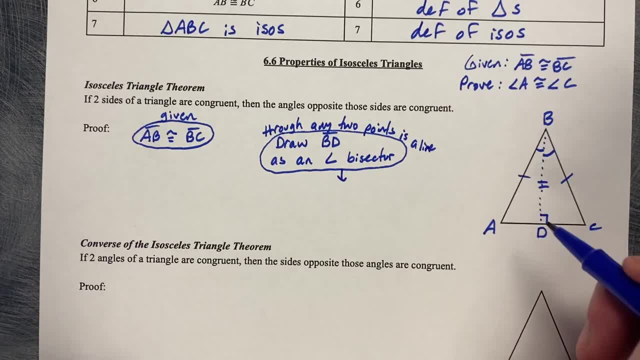 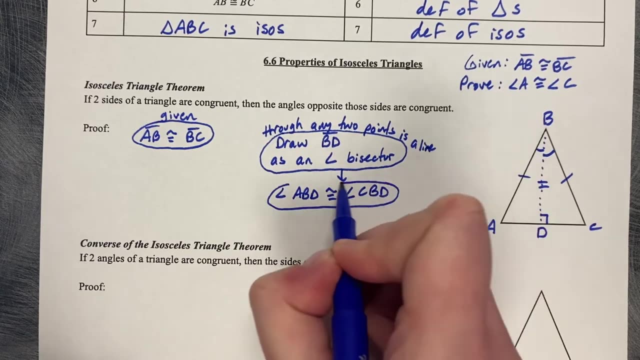 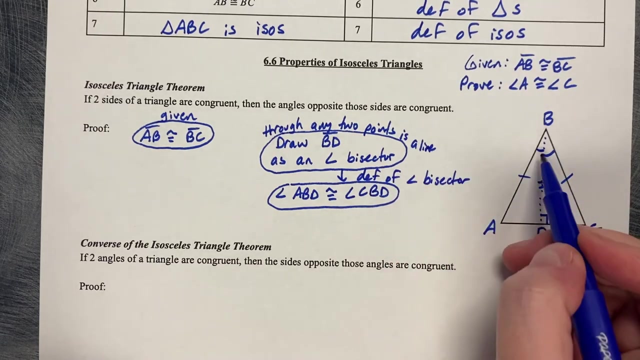 So now if those two, if that's an angle bisector, then we can say that those two angles are congruent. So we can say angle ABD is congruent to CBD, And that's by the definition of angle bisector. So now I've got my angle and then now we need to say: 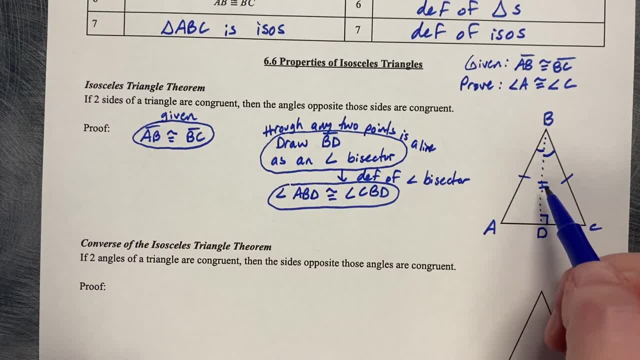 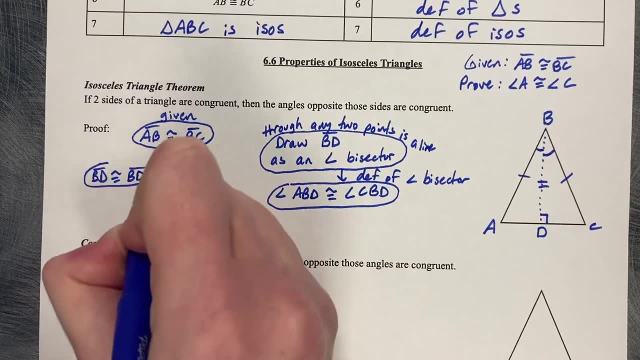 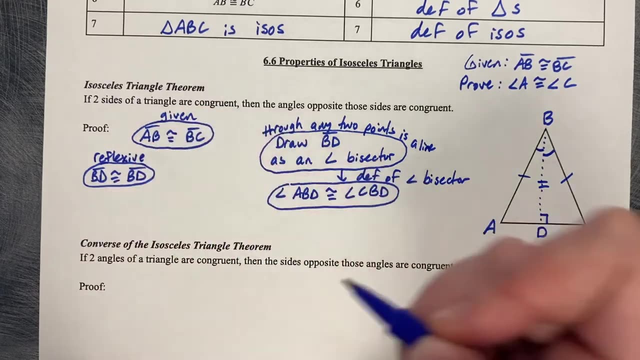 and then I've already got these two sides, but then I just need this last side. We've done it a bunch of times, I'm going to do it over here. BD is congruent to BD. It's a shared side, So you could say shared side or reflexive property. 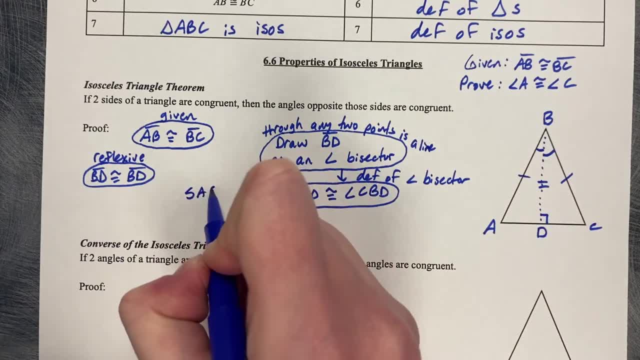 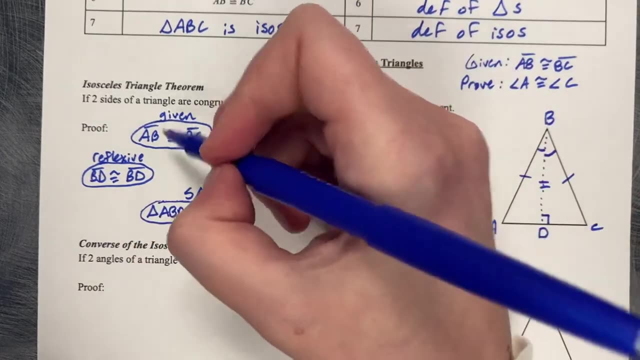 And so now we can bring those together using side angle side. We can say that triangles ABD is congruent to triangle CBD, So that's by a side angle BD. And then we can say that triangle ABD is congruent to BD. 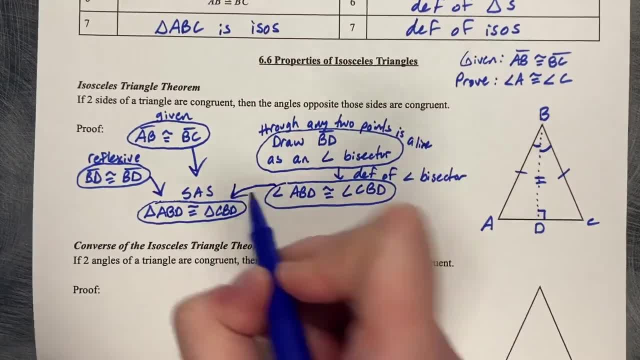 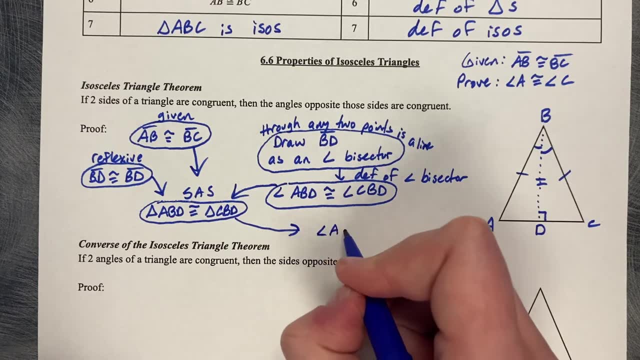 So that's by a side angle BD. So that's by a side angle BD. So that's by a side angle BD And that side and an angle, And then our final step here is: because those two are congruent, then we can say: angle A is congruent to angle C. 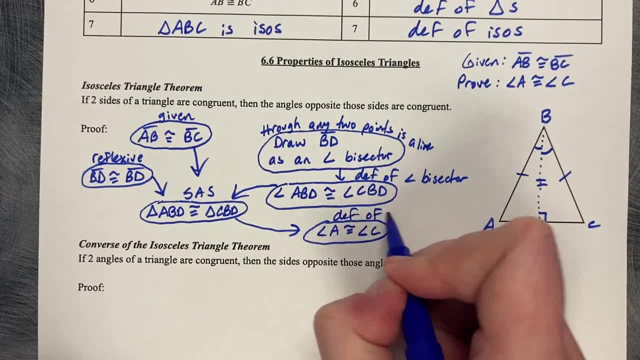 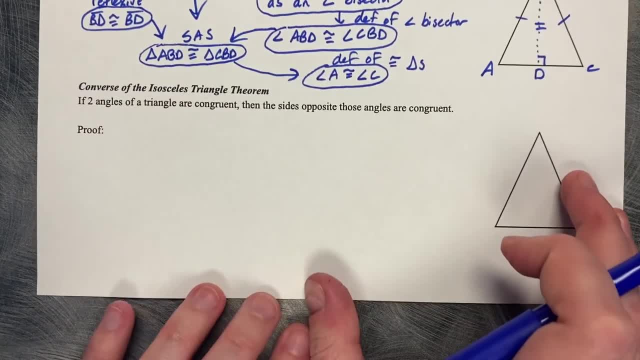 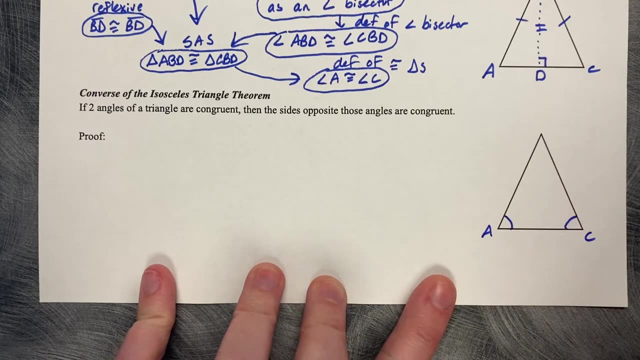 It's our final piece and that's the definition of congruent triangles. You can also go the other direction. So in this one it says: if two angles of a triangle are congruent- so we've got our angle A and angle c are congruent, then the opposite sides of those angles are congruent. so what you would do, 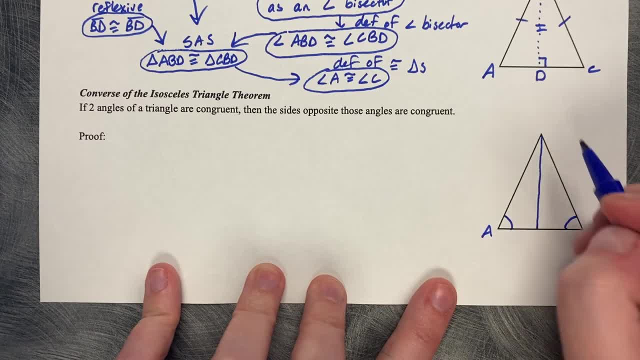 is you draw in your height or altitude. again, make it an angle bisector. let's do two tick marks on that, because i did one down below, and then you would use the shared side length. so in this case it would be angle angle side. so i'm actually not going to write the whole proof, but you would do. 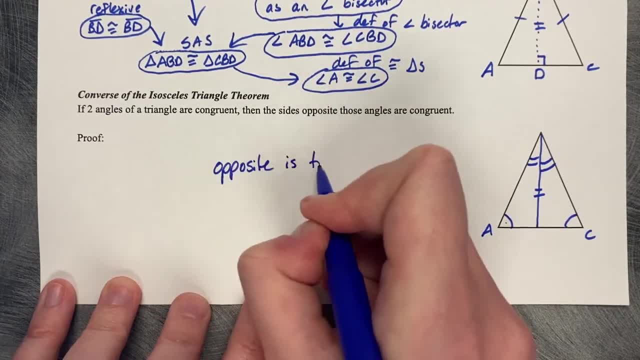 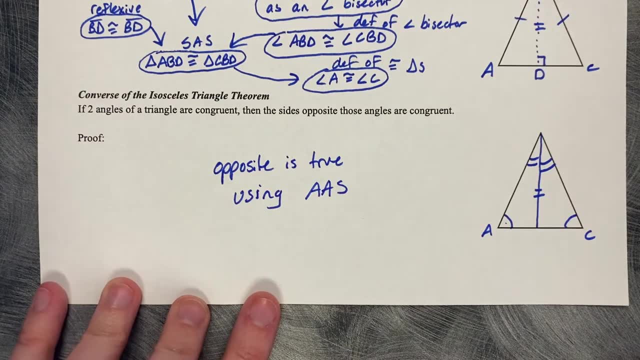 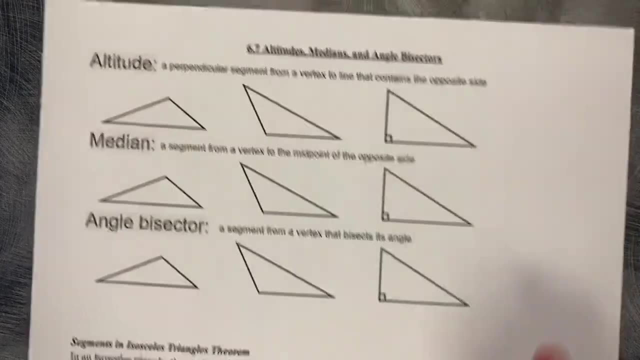 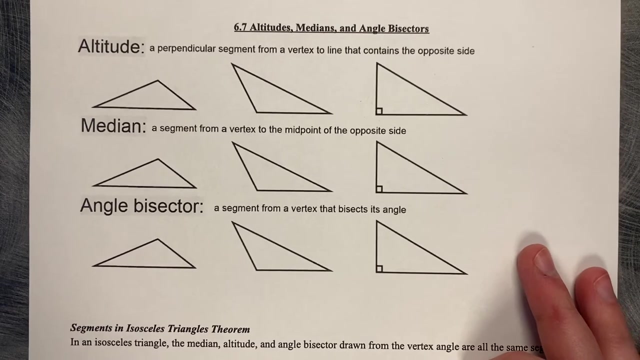 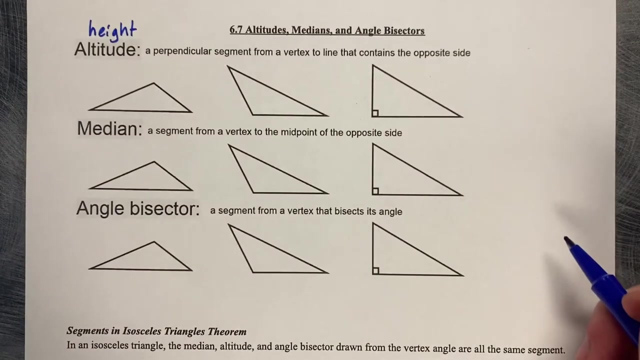 the opposite is true, using angle angle side instead of using side angle side. all right, 6.7 altitudes, medians and angle bisectors. so first thing we're going to talk about is an altitude. the synonym for altitude is also height, and, and If you find the height of a triangle, you have also found the altitude. 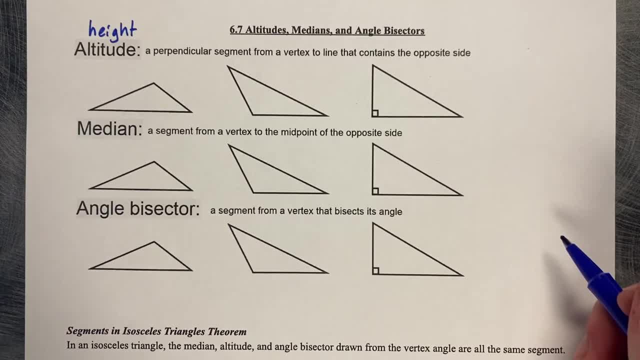 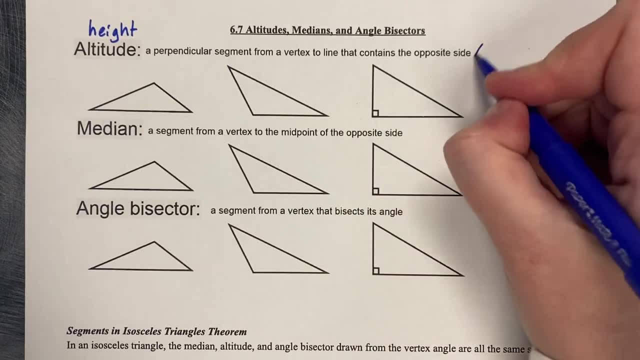 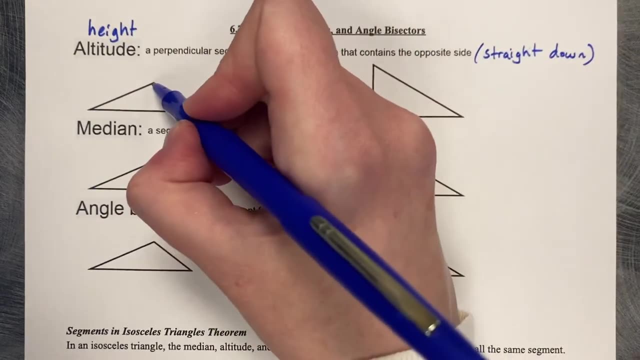 So in your mind, make sure that you know that those are interchangeable with each other. So it's a perpendicular segment from a vertex to a line that contains the opposite side. So straight down is how I like to think about it. So in this one I go straight down, perpendicular. 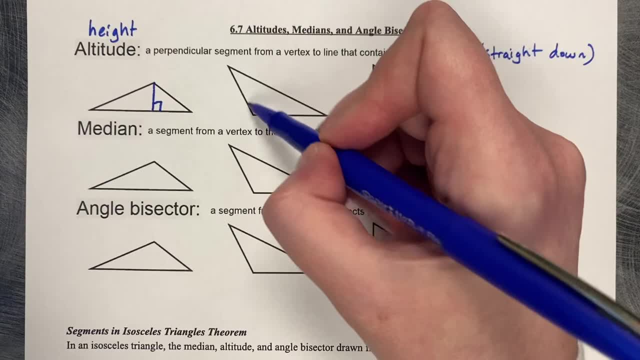 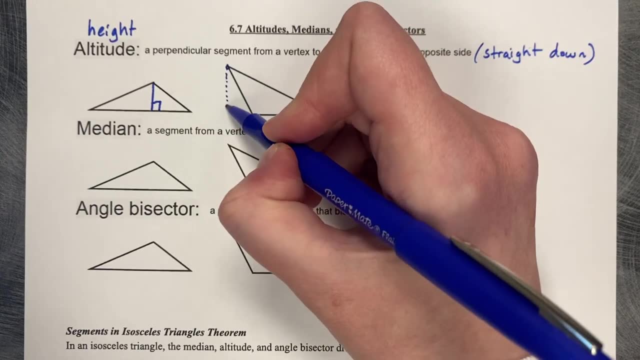 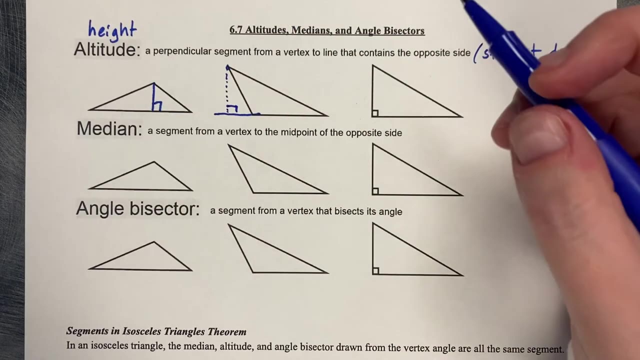 You can. also, if it's an obtuse angle like this, sometimes the altitude lies outside of the triangle. So from this vertex straight down actually hits outside of this triangle and that's okay. It's still the height, but it's outside of the triangle. 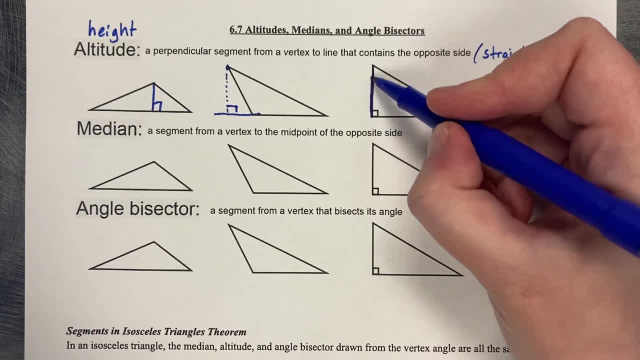 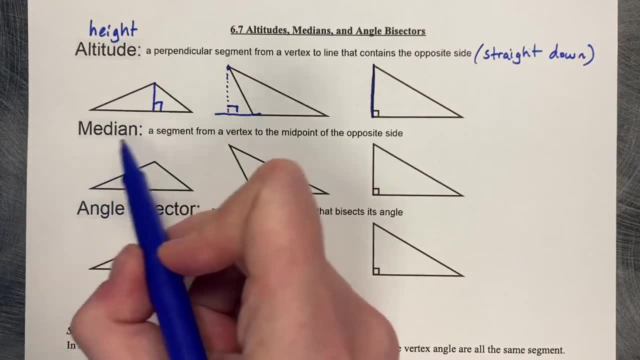 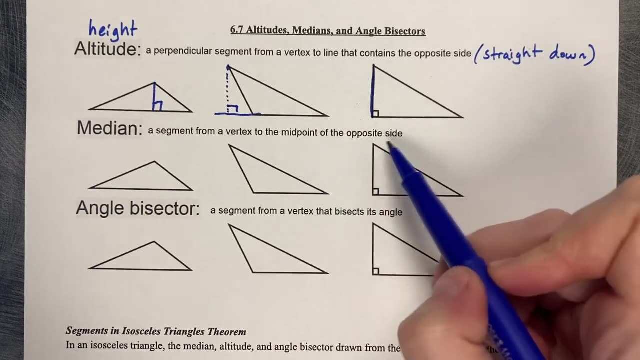 On a right triangle here. if it's upright like that, then straight down is your perpendicular. so that is your altitude. Medians, Median or the preamplifier Prefix med, need is middle, So a segment from a vertex to the midpoint of the opposite side. 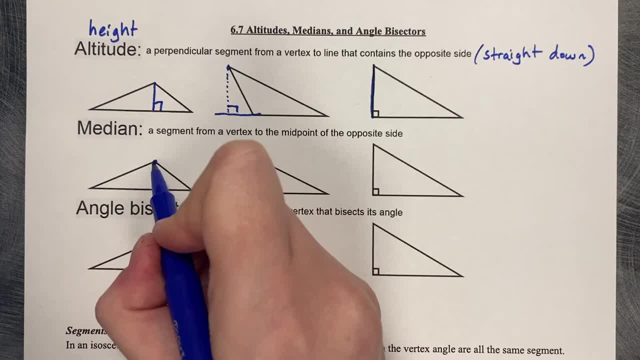 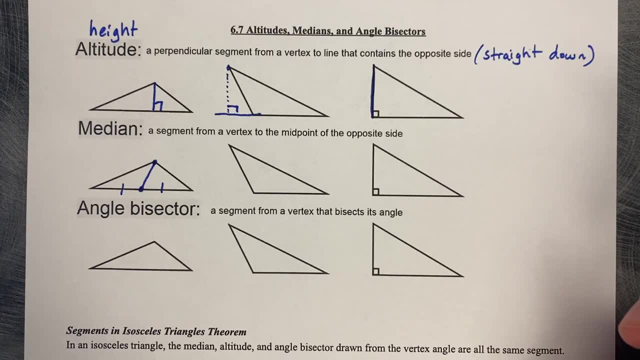 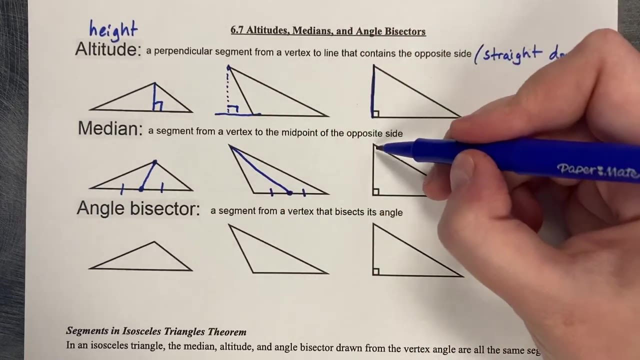 So you're going from this vertex to the middle of the opposite side, and then you can use tick marks to show that those are now congruent to each other. So from the vertex to the middle, From the vertex to the middle, You can do it from. 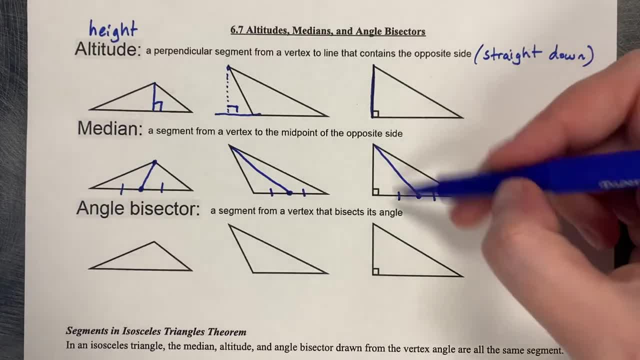 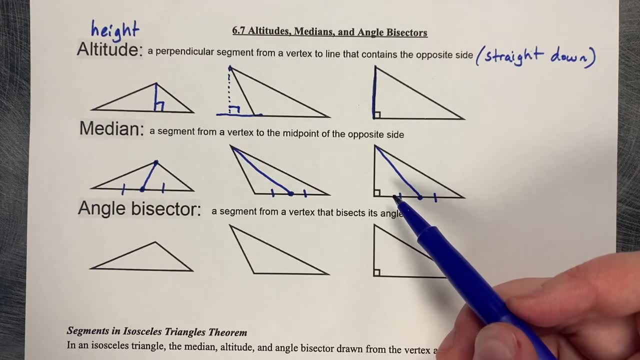 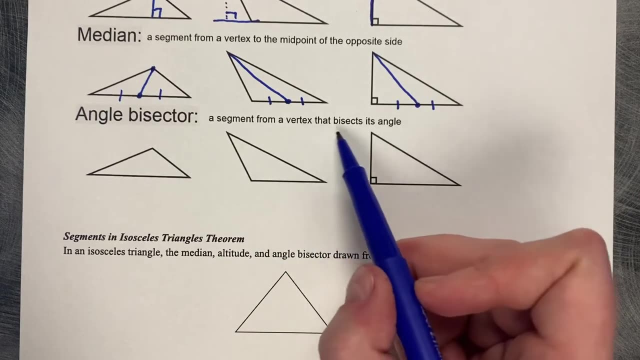 Other side links as well. If you do all three of them together, if you do three medians together, it creates an intersection called a centroid, And that centroid is the center of gravity. So check that out too. Angle bisector is a segment, that, a segment from a vertex that bisects its angle. 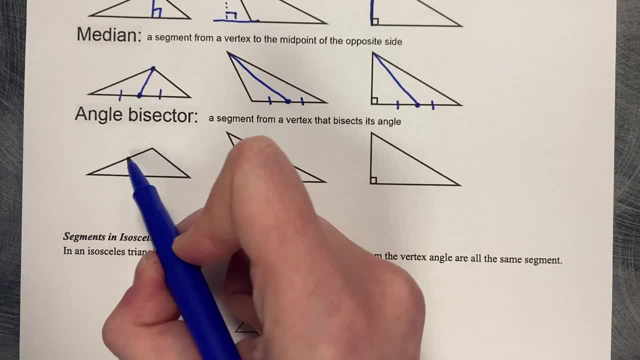 So what you're trying to do is focus your eyeballs on the angle and cut that angle in half, And I like to do a full length arrow on it. I know it, It looks like a bisector, It's almost a bisector, but it's not a bisector of the side length. 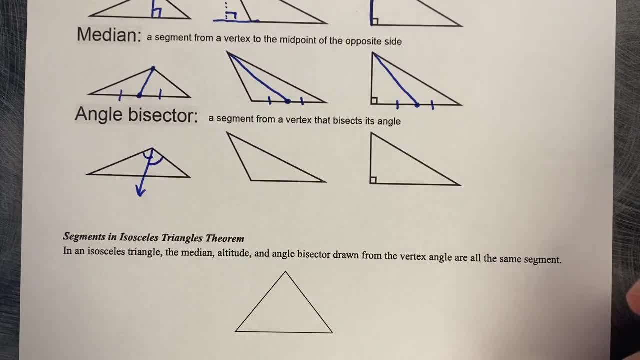 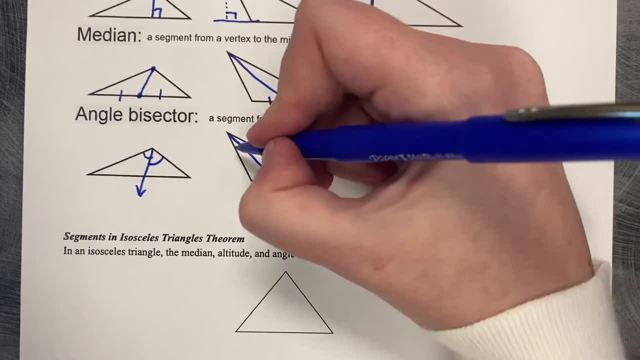 It's a bisector of the angles up top. So on this one again, you're looking at this small acute angle and cut that angle in half. See how that one is less of a bisector on the opposite side length. So just be careful. 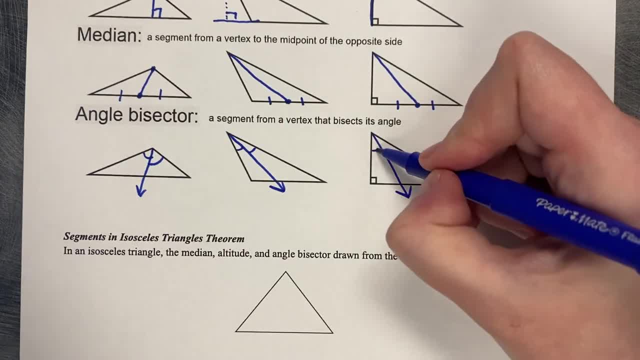 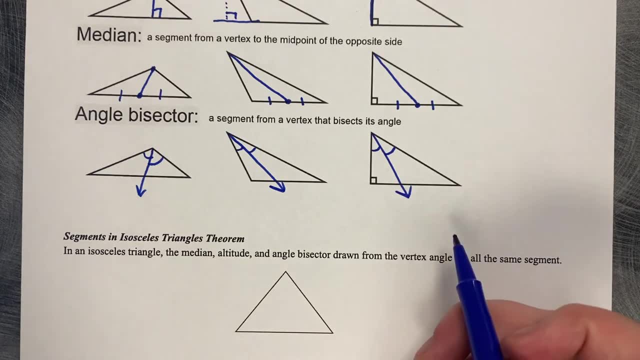 All right, We're trying to do a bisector on this one. Again, on that one, it's not the bisector, It's the angle bisector, Not Not the segment bisector. Okay, Segments and isosceles triangles theorem. 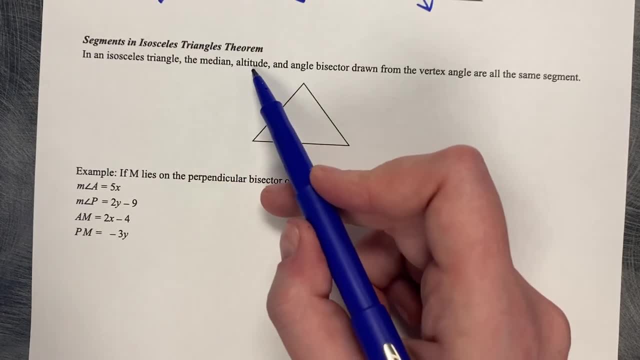 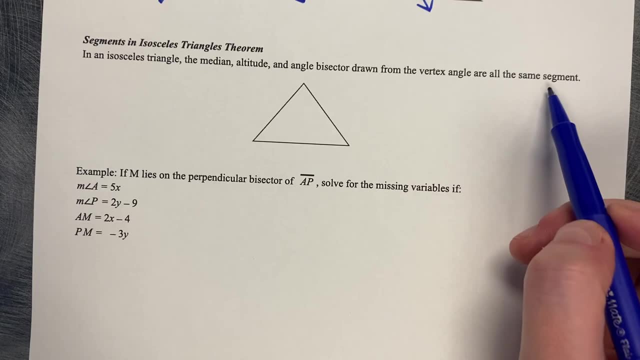 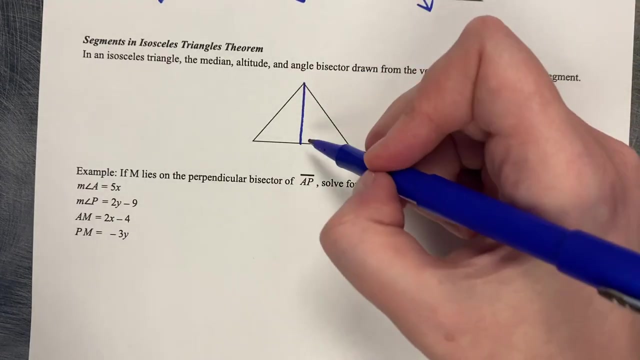 This is the one I was saying before. In an isosceles triangle, the median, the altitude and the angle bisector, the same line drawn from the vertex, are all the same segment. So if I draw the angle bisector, the perpendicular bisector and the median, those are all three the same line. 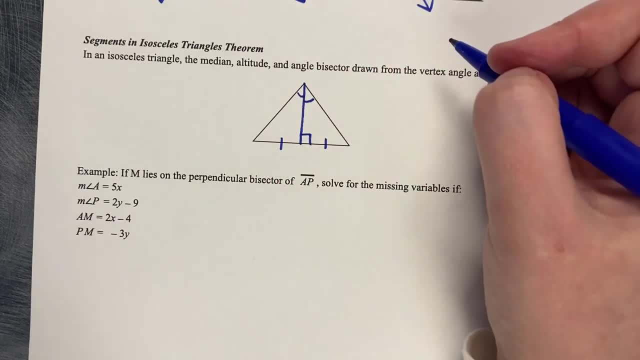 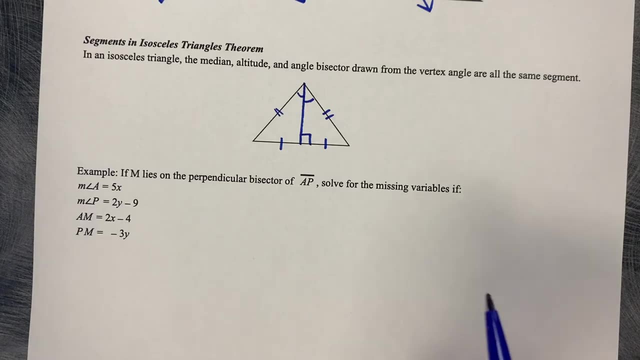 So that means that this angle Is congruent to this angle And you've got this side congruent to this side Because it's an isosceles triangle. So that line is the same one for isosceles triangle. It's a median altitude and angle bisector. 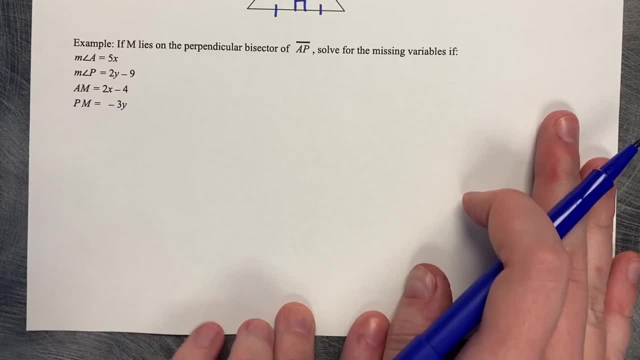 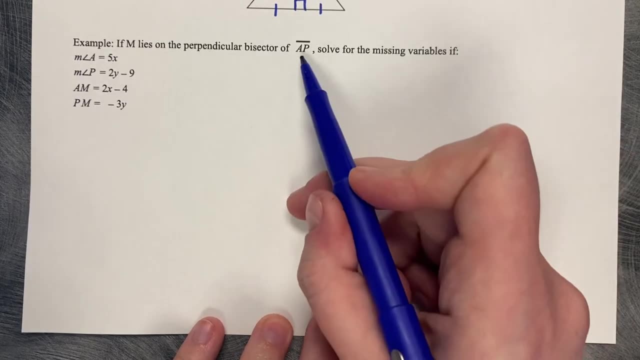 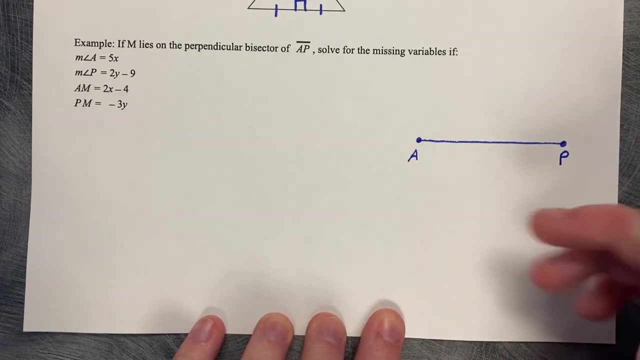 All right, Our last example: If M lies on the perpendicular bisector of AP, solve for the missing variables. So let's give ourselves a diagram. So we're talking about the segment AP, And then we want M to lie on the perpendicular bisector. 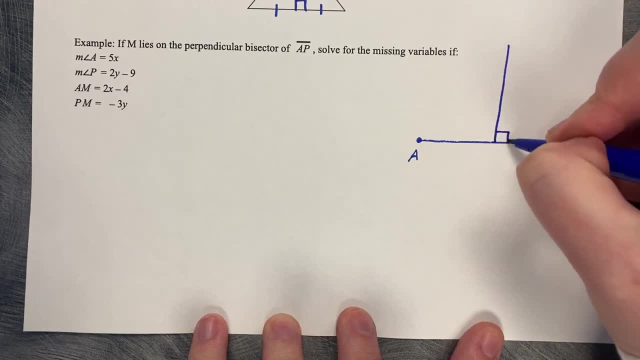 So perpendicular And it's a bisector, So that means that these are the same here. And then we want point M on this perpendicular bisector. So choose any spot. I'm just going to choose it up here. There's M. 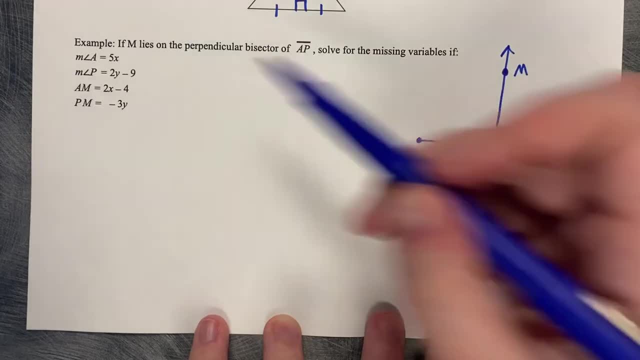 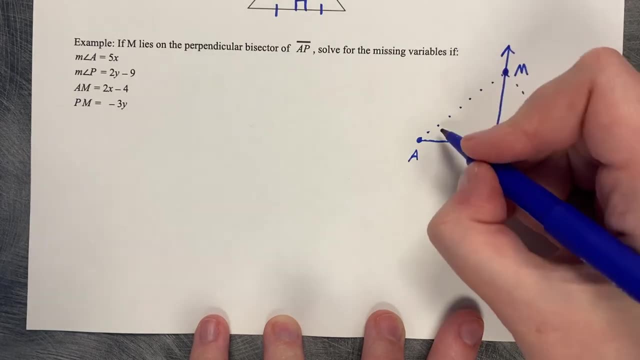 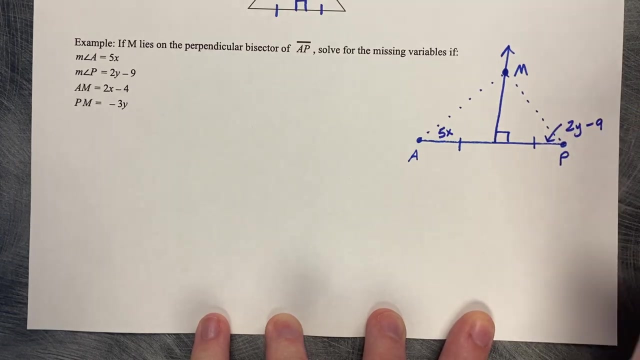 So We've got some information about AM, PM, angle A and angle P, So I'm going to connect these up. So it's saying that angle A is 5X, Angle P is 2Y minus 9.. AM is 2X minus 4.. 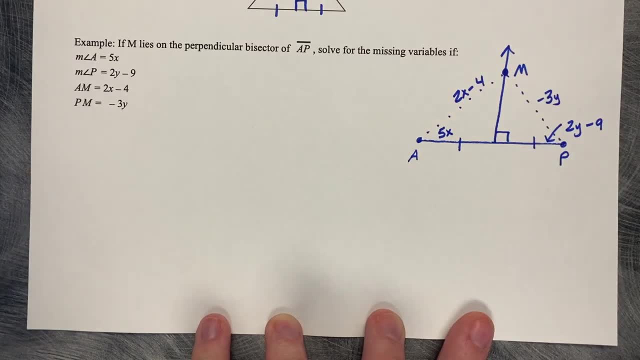 And PM is negative 3Y. So if you take a look at this, you can see that if these are congruent- And this is a perpendicular bisector- Then the length of AM must be congruent to the length of MP. We know that because this is for sure a perpendicular bisector. 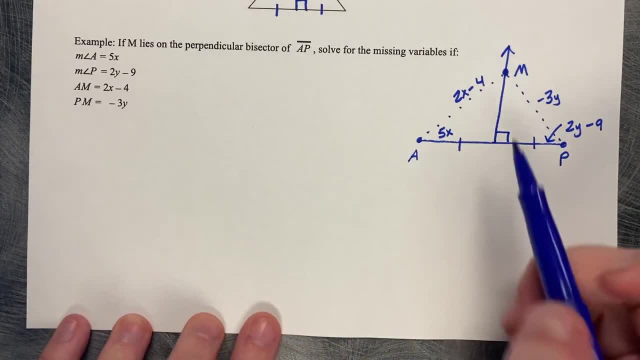 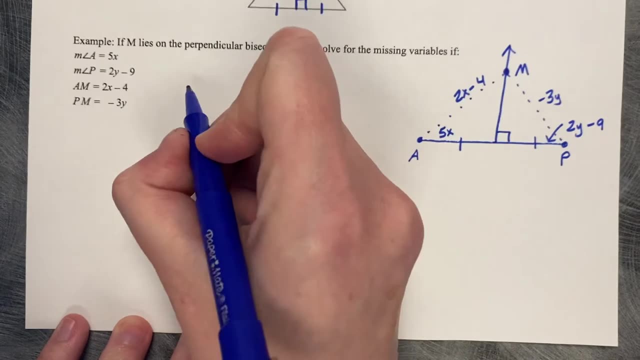 They told us up top. So what we can do is we can set some stuff equal to each other. So that means that this is an isosceles triangle, Which means that angle A is going to be congruent to angle P. So we can say: 5X equals 2Y minus 9.. 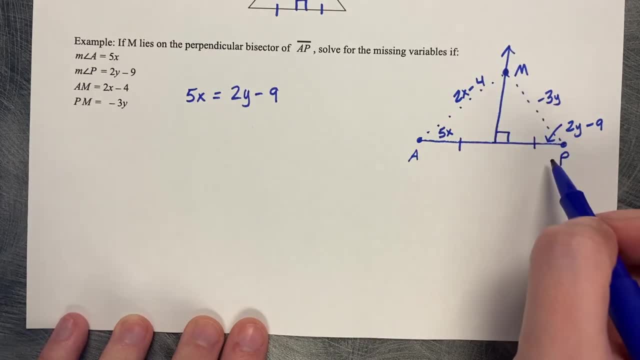 We can also say that AM is congruent. It's congruent to MP, So 2X minus 4 is equal to negative 3Y. Now I've got two equations and two variables, So we're going to use systems of equations to help us solve this. 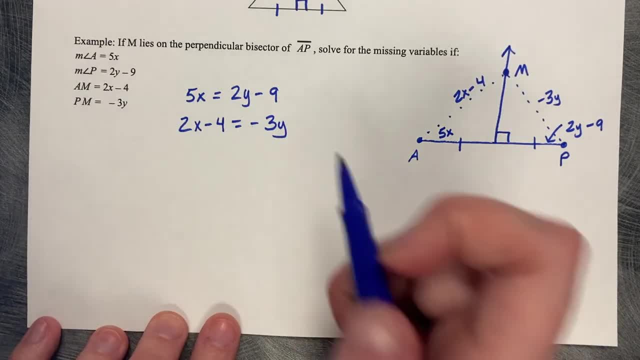 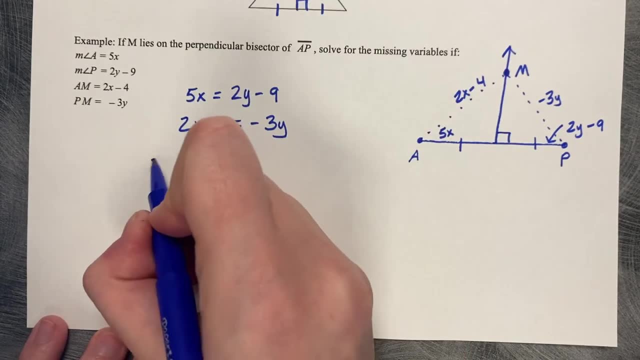 I'm going to go for elimination. You could go for substitution. You're pretty close to substitution here, But I'm going to go for elimination, So I'm going to get them in standard form. So I want 5X on the left. 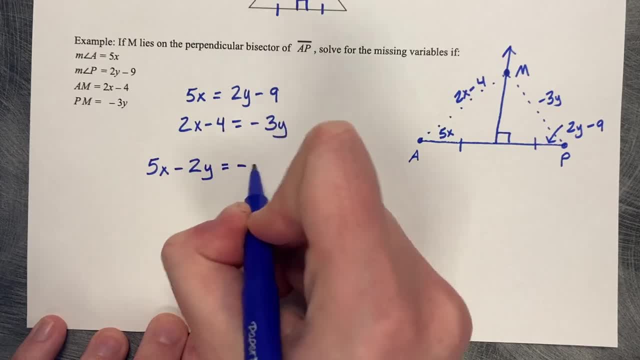 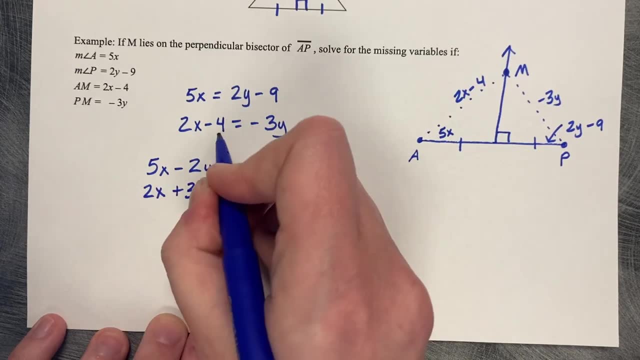 But I also want the Y on the left. So minus 2Y equals negative 9.. 2X: Bring the plus 3Y over And add 4.. So I did that in my head. I think I'm going to cancel the 2 and the 3 using a 6.. 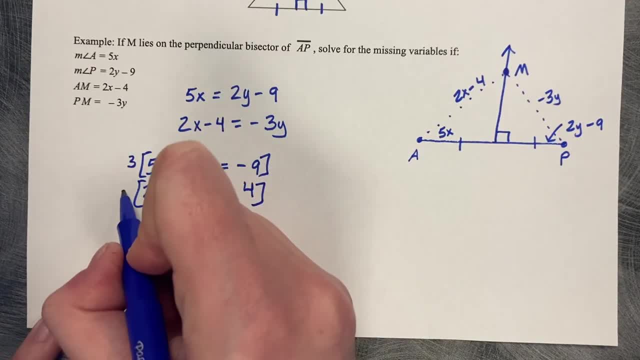 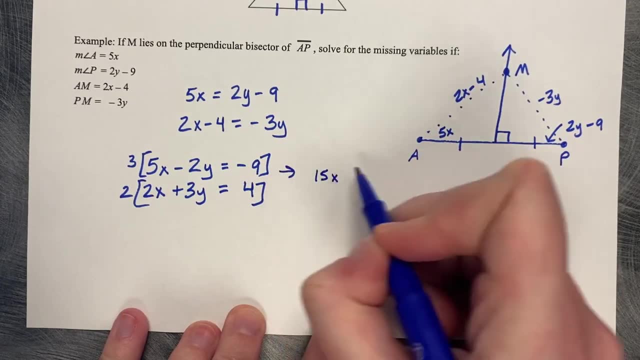 So I'll multiply this one by a positive 3. And this one by a positive 2. Because this is a negative 2. So then, coming over, we've got 15X minus 6Y equals negative 27.. 4X plus 6Y equals 8..